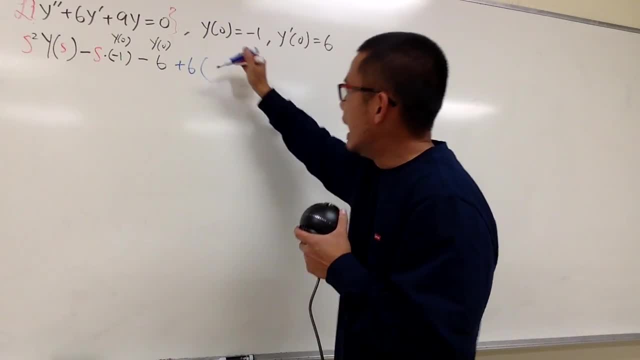 For y prime. we will end up with what S times? let me just write it down: better s times: y of s and then minus. let me just write it down: minus y of 0,, which is negative 1.. 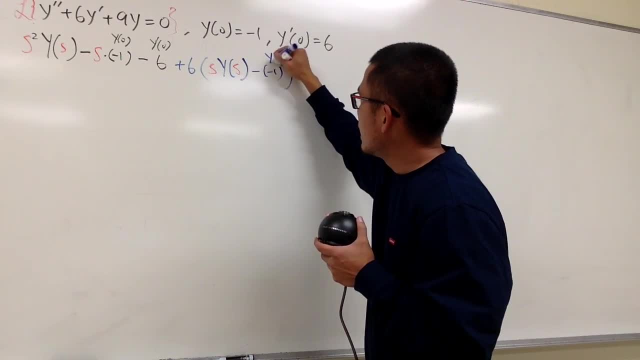 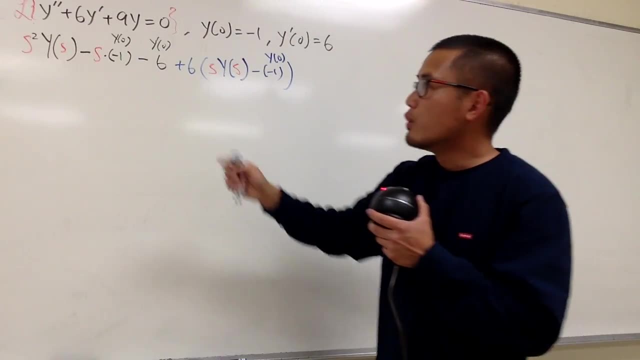 So let me just indicate this right here is negative 1.. Like this, this is y of 0, right, So the blue portion is for the middle term. right here At the end, we have plus 9y, so we have plus 9.. 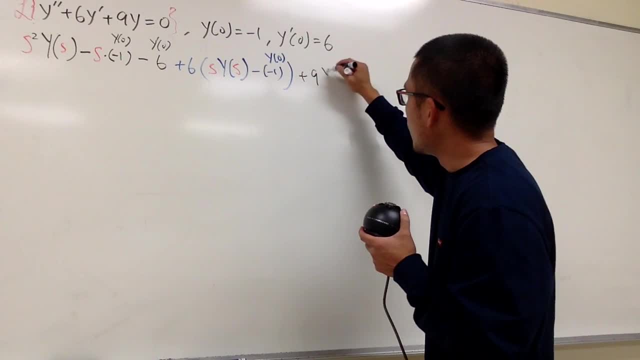 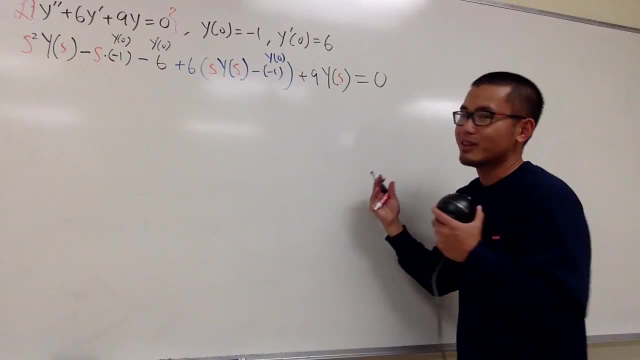 And then, once you do the Laplace transform of y, you get y of s like this: And we are lucky because the right-hand side is just 0, so we just have 0 right here. So far, so good. And now the usual deal is that we have to get all the ys right. 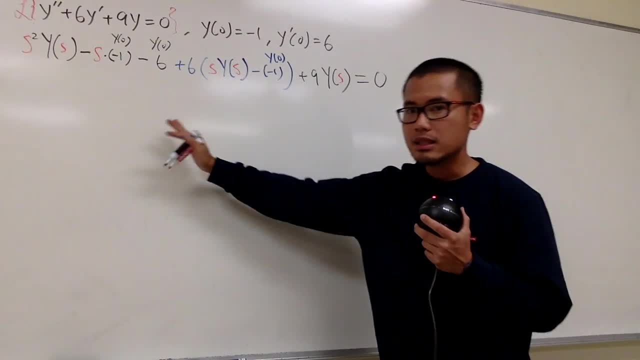 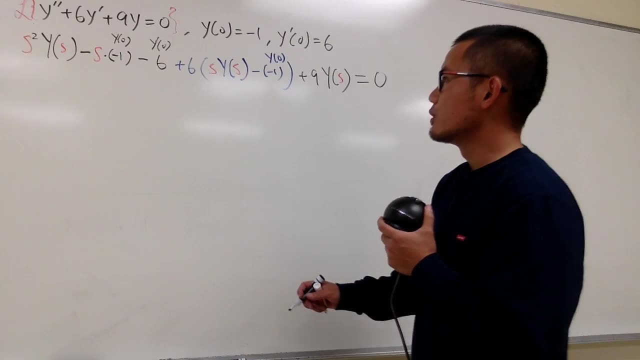 And then collect like terms And we want to isolate the ys on the left-hand side and then put everything right here on the right-hand side. So perhaps let me just do one more step. Let me just clean things up to make it easier to understand and follow. 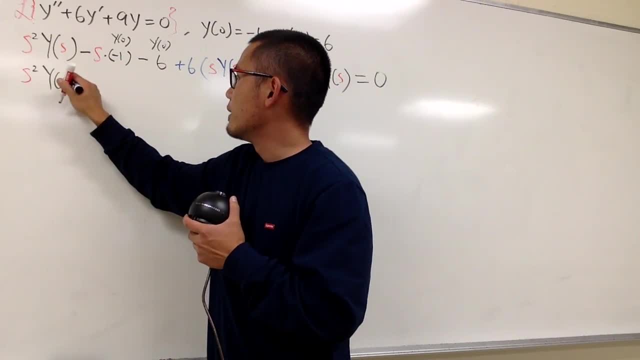 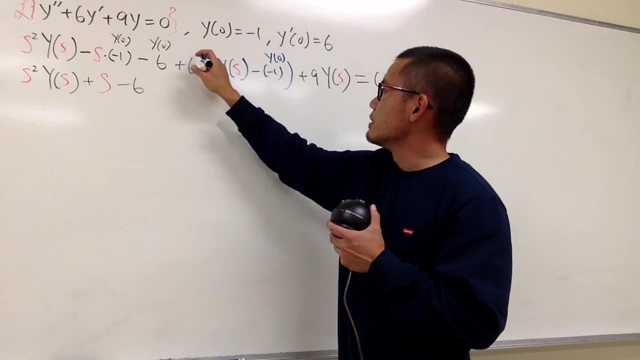 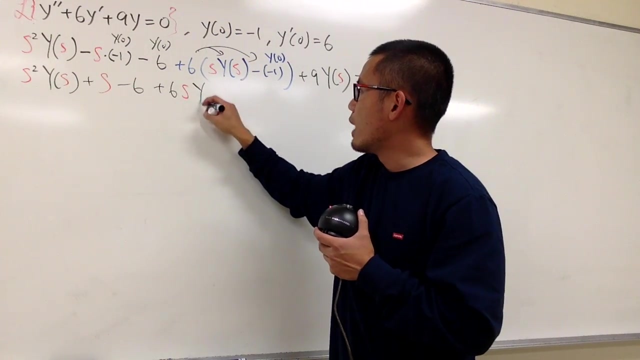 This is s. So we have y of s squared, and then we multiply by y of s, And then this, and that becomes plus s, And then this is minus 6. And here I will have to distribute right. So this is 6 times that. so it's plus 6s, and then y of s. 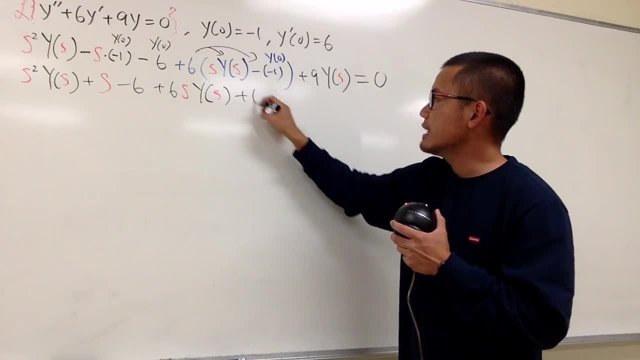 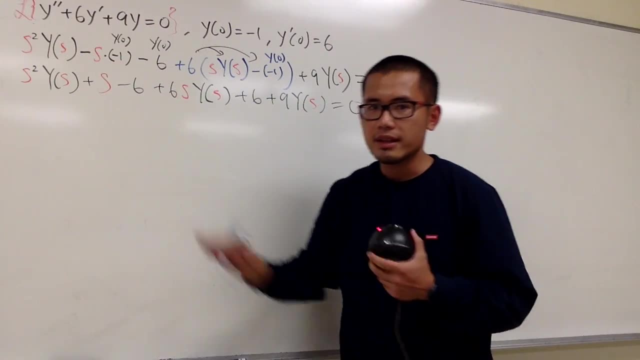 And then 6 times that this is negative. negative it becomes positive, so plus 6.. And then this is plus 9 times y of s And you see All my s are in red. No 5, right. 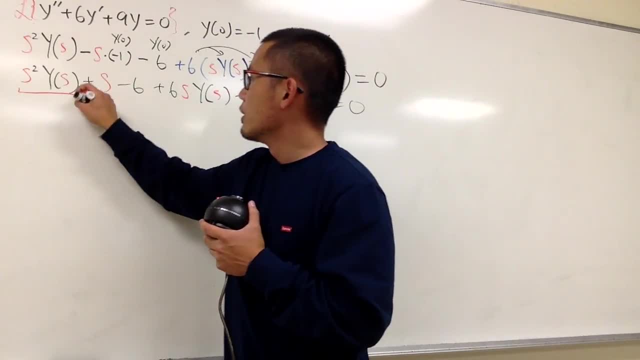 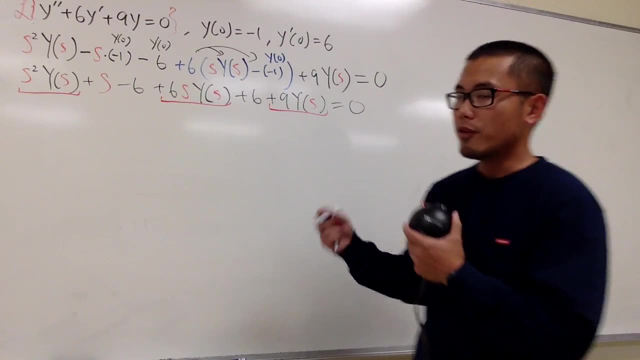 And now let's see, what do we have? Here we have the y of s, and then here we also have the y of s, and here we also have the y of s. We will put them together and we'll factor out the y of s right. 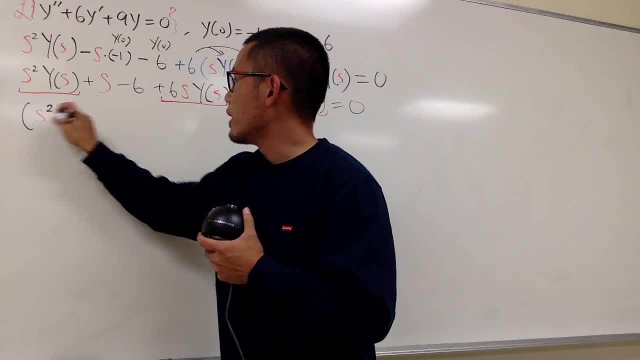 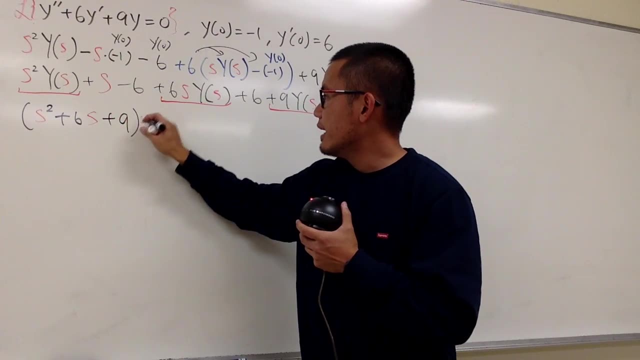 So, as we can see we have, here is s squared, and then this is plus 6s, and then plus 9, right here, right, And then we multiply by y of s right here, And we bring everything else to the right. 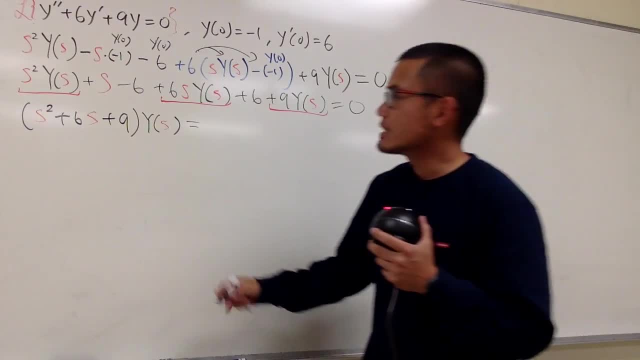 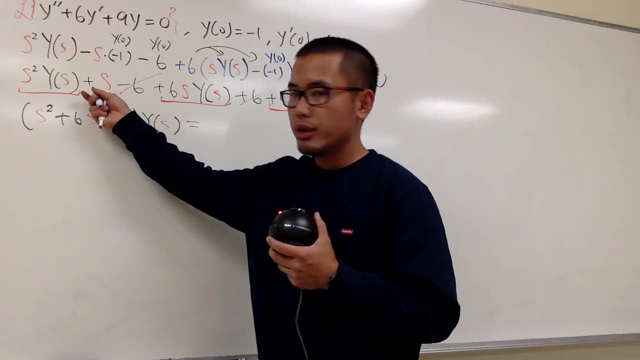 We bring everything else to the right-hand side And notice that the minus 6 plus 6, they cancel each other out, which is excellent. I will just have to bring the s to the right-hand side, So it becomes negative s like that. 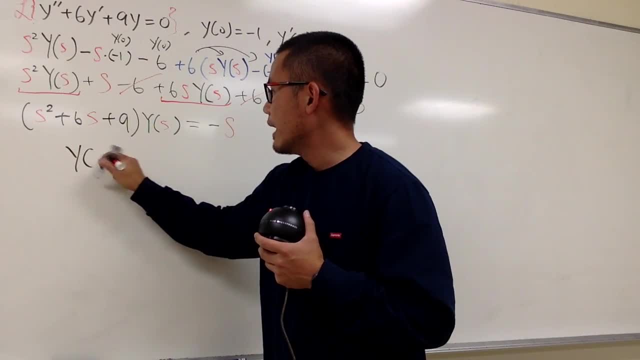 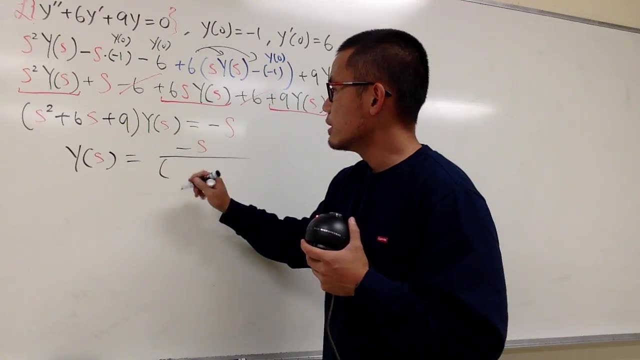 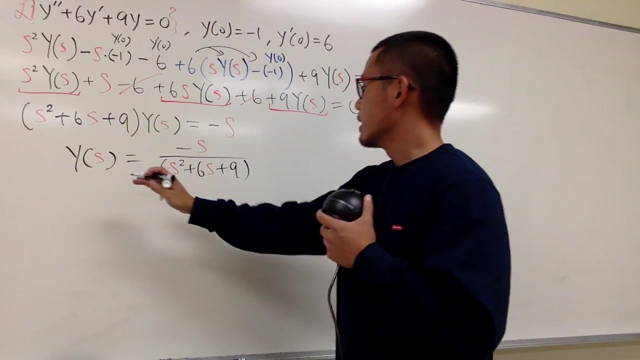 And at the end you will see, we will have y of s which is equal to. this is negative s on the top over this, which is parentheses s squared Plus 6s plus 9.. That's it right. 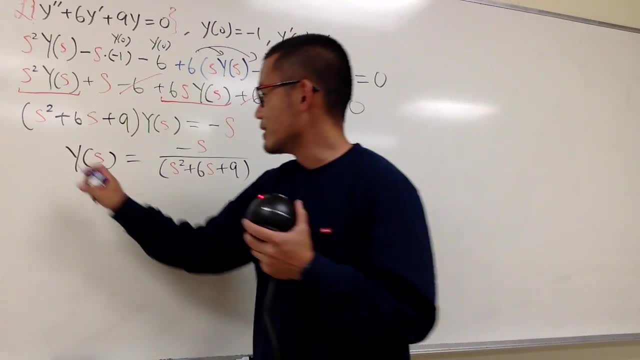 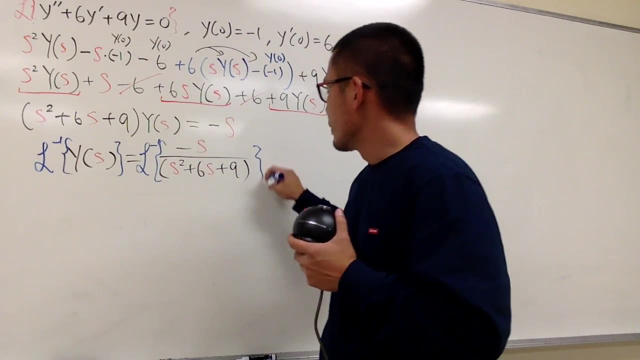 And to get back to the t-world, we have to do the inverse of the plus, and let's do so on both sides. So on the right-hand side we'll get y of t, and that's the solution to this initial value problem. 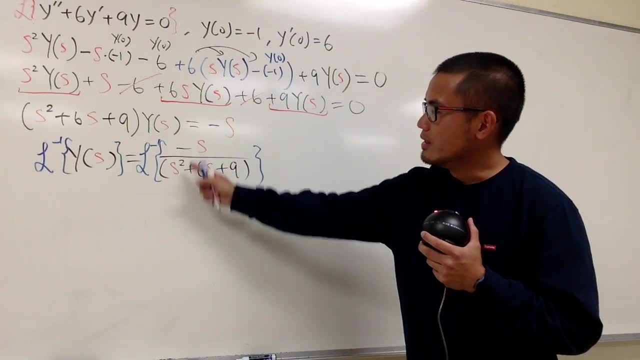 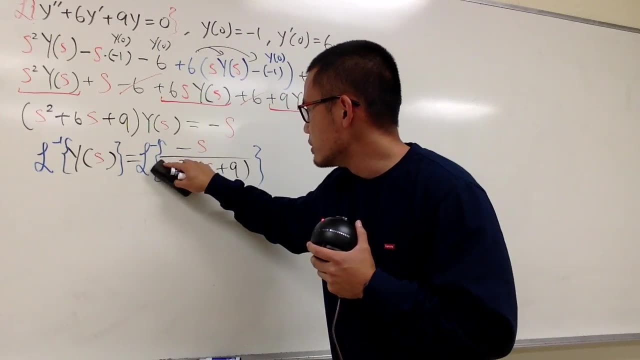 And now here's the deal. How are we going to get this right here? right, The inverse of the plus of that, Perhaps. let me not use the parentheses right here, Let me just write it down. That's how it is. 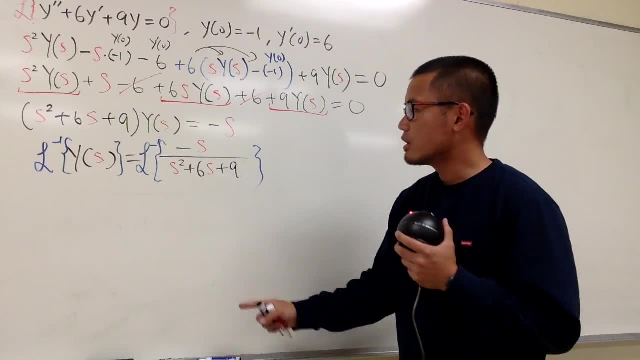 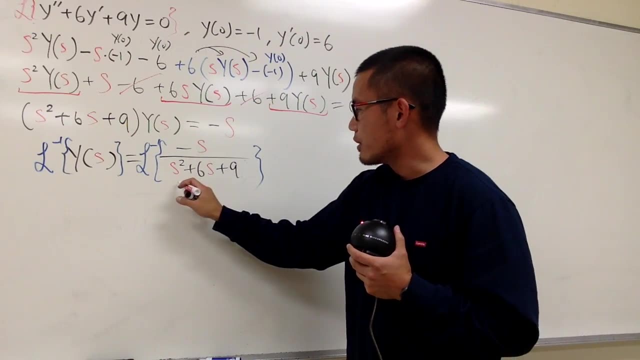 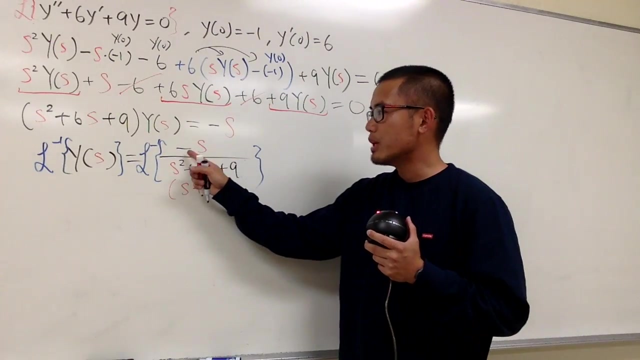 Well notice that on the denominator we have what This is: s plus 3 squared. right. We can factor it out. So let me indicate that right here, This is just s plus 3 squared Well. unfortunately, on the top we have a negative s. 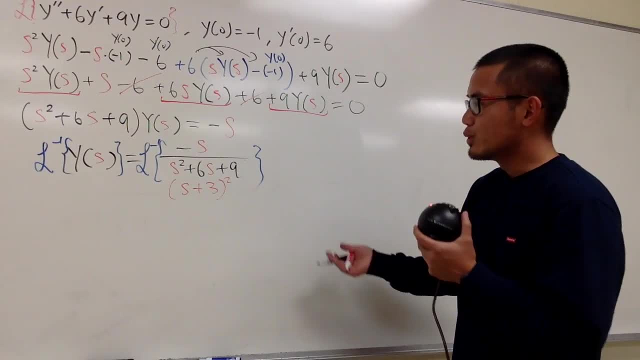 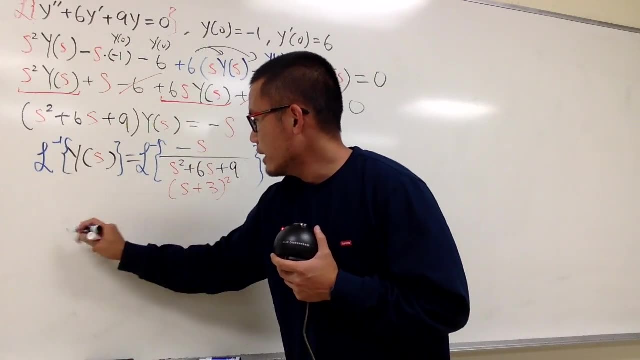 So this is not real quick right away, But we can still do it with a reasonable amount of work. Let me show you So: on the left-hand side it's just going to be y of t, and this is the solution to the initial value problem. 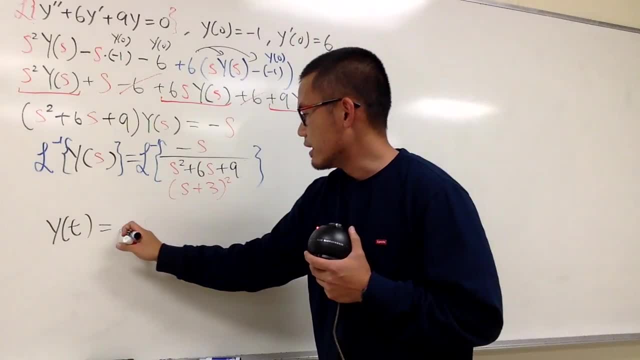 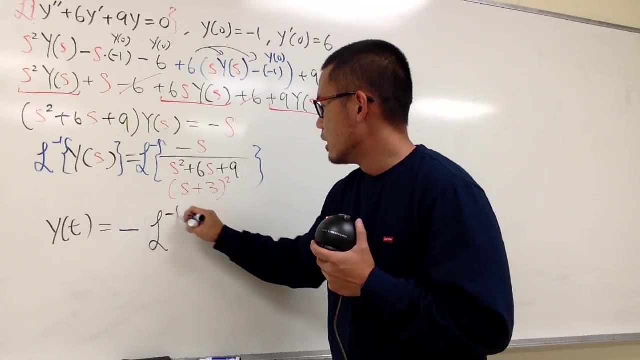 And let me bring the negative to the front. So we have negative right here And right here. let me just write it down as the inverse, not plus. On the top we still have s. On the bottom we have this s plus 3.. 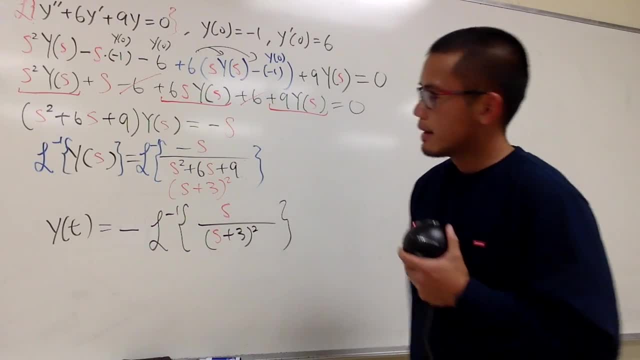 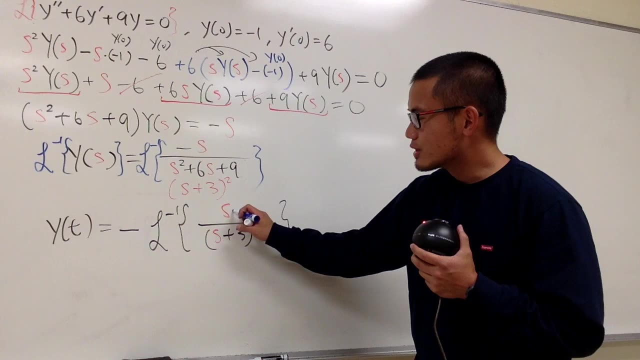 And then square. And now you have choice. You can do partial fraction, the good old-fashioned way, or I can just go ahead and plus 3 to this, because I can match this and that and you can cancel things out. That's really nice. 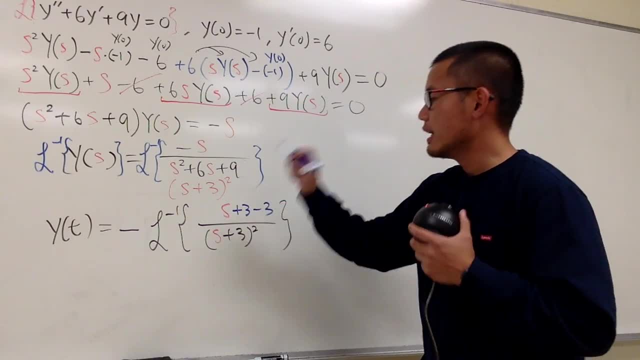 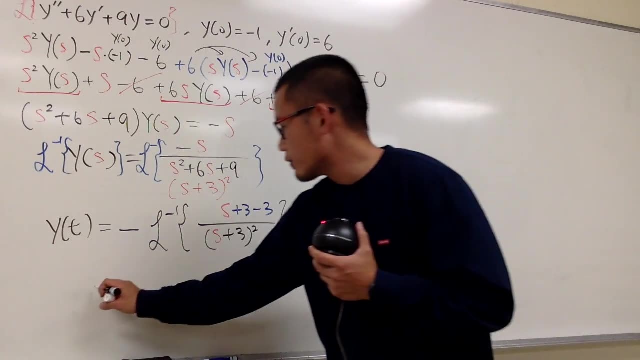 However, after you plus 3, be sure you minus 3 as well. And don't forget, you still have this negative all the way in the front. all right, And now let me just continue by doing so for you guys: Negative all the way in the front. and then the first thing is just going to be: 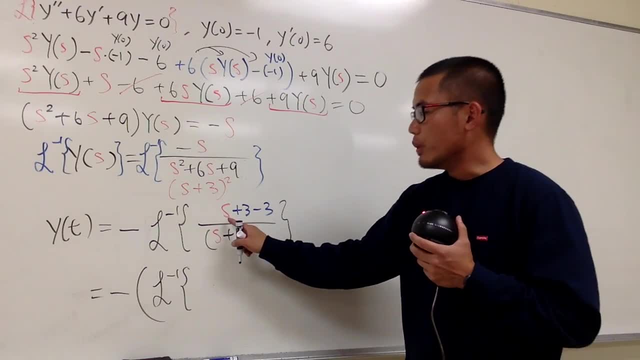 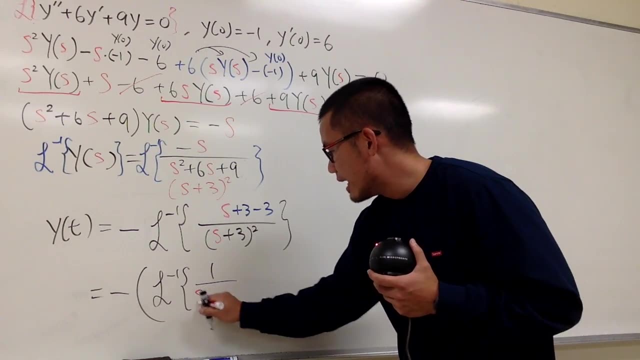 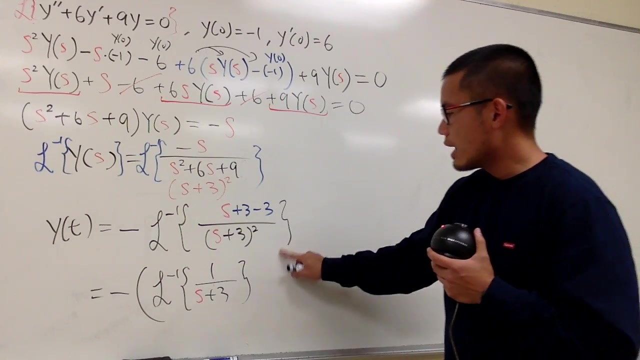 let's look at the inverse, not plus. We have s plus 3 over s plus 3 squared, So that will be just 1 over s plus 3 to the first power. all right, And I'll close this right here. And for the second one we will have: 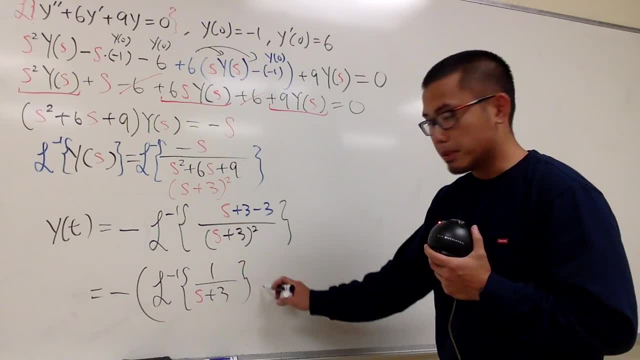 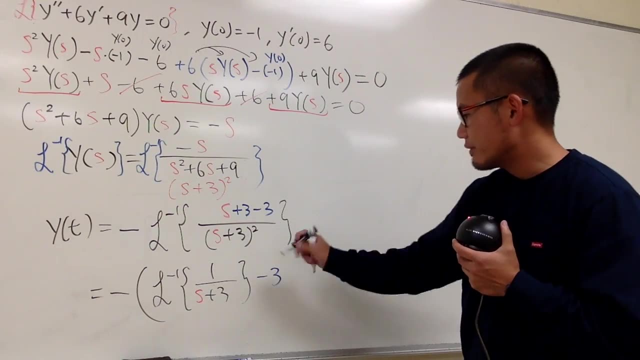 I've put down the negative all the way in the front already, so technically it will be plus, but this is negative 3.. I would like to take that to the front. so we have negative 3 right here And then we have the inverse, not plus. 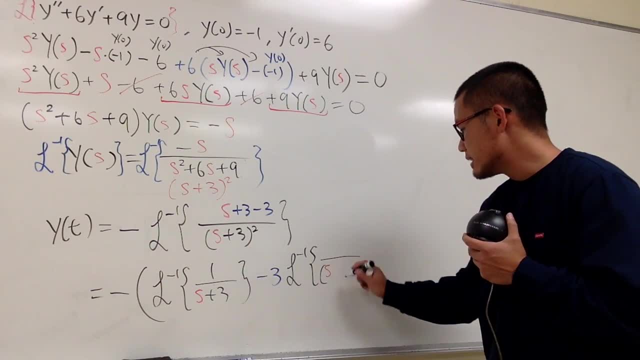 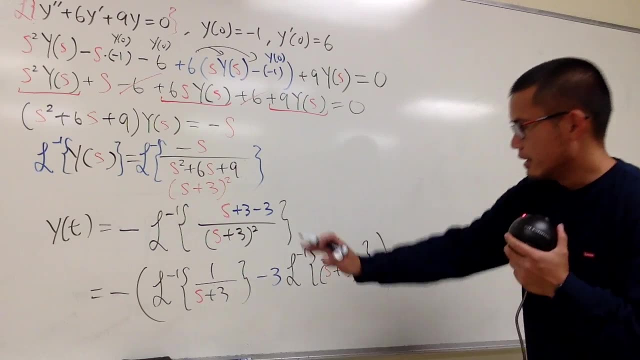 On the bottom, it stays the same s plus 3, like this squared, and we can put down 1 on the top. Okay, this is what we have at the moment. We can totally take off this. And how about this right here? 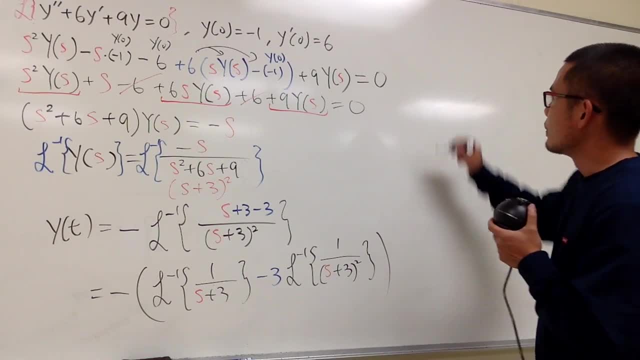 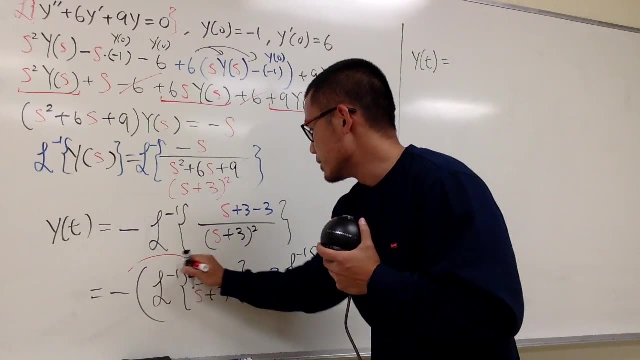 We should also be able to do so as well, right? So let me just write it down right here for you guys. y of t is going to be first of all, perhaps let me just distribute the negative into the parentheses, for you guys. 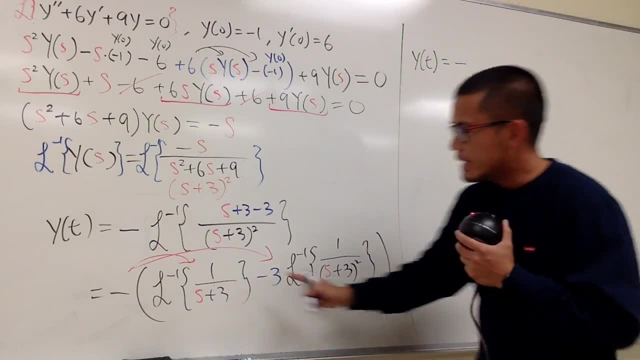 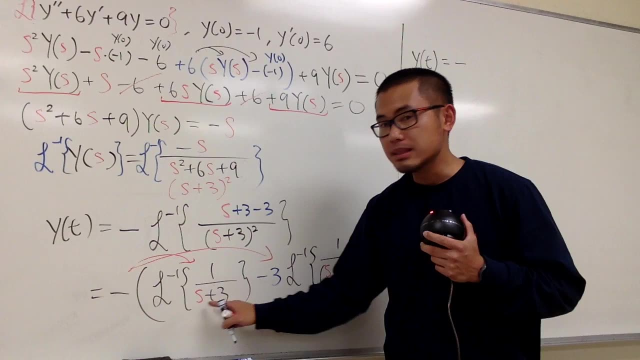 So we will have negative and for this- right here, we know it's going to be what- e to the negative 3t, because this is 1 over s minus negative 3,, right, So e to the negative 3t, like that. 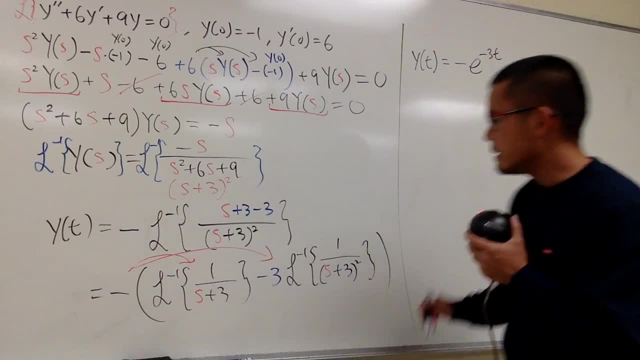 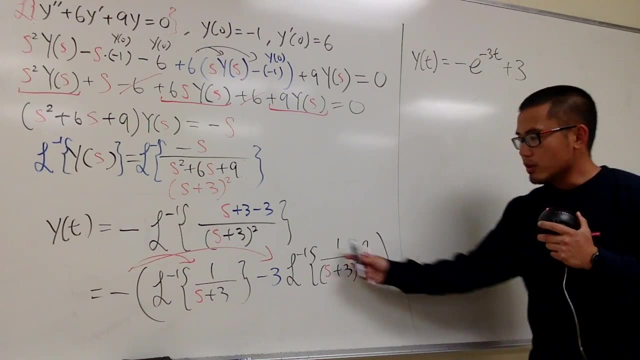 That's it. And then negative times, negative becomes positive and then, if you would like, you can have the 3 right here. Let's put that down, all right, How can we take off this? Look at the 2 as 1 plus 1, right. 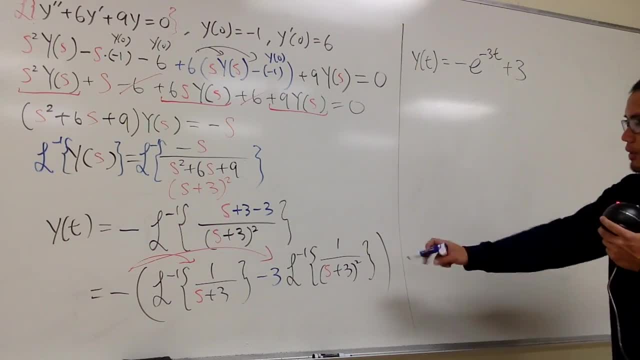 So I'll put this down in blue on the side For that one, the inverse dot plus of that, which is 1 over s plus 3, look at that as 1 plus 1.. And you know, this one will tell you the nth value.